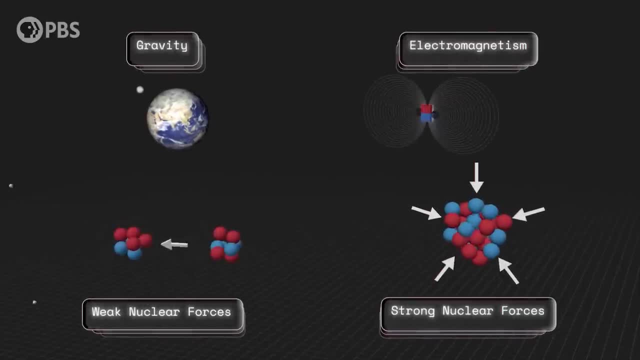 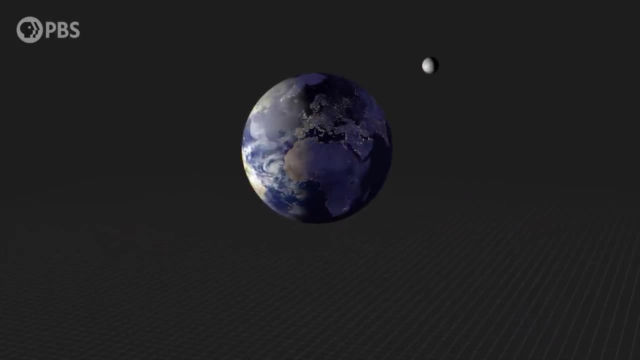 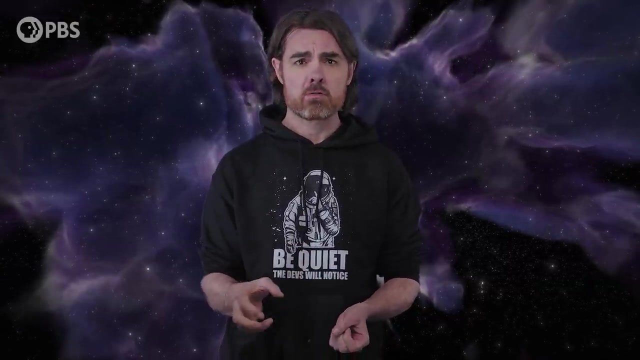 We're told there are four fundamental forces: Strong and weak, nuclear forces, electromagnetism and gravity. Except maybe gravity is actually no more fundamental than, say, the force of a stretched elastic band. Maybe gravity is just an entropic byproduct, an emergent effect of 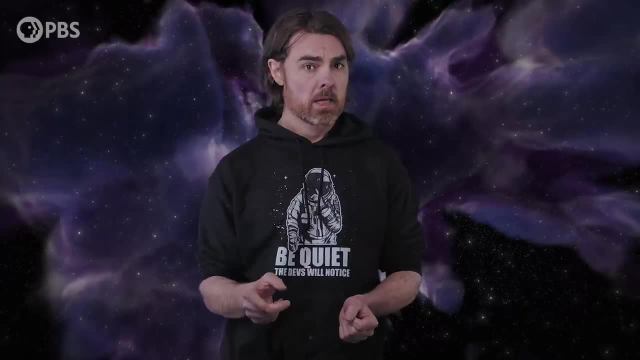 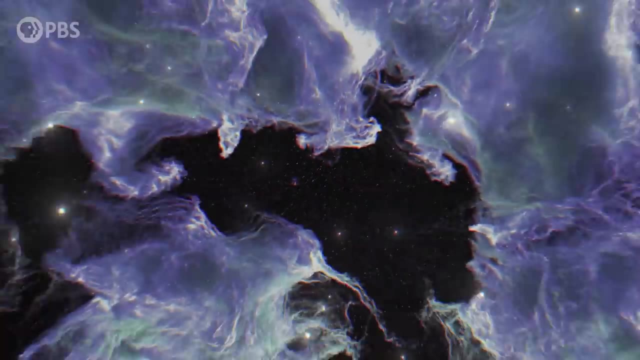 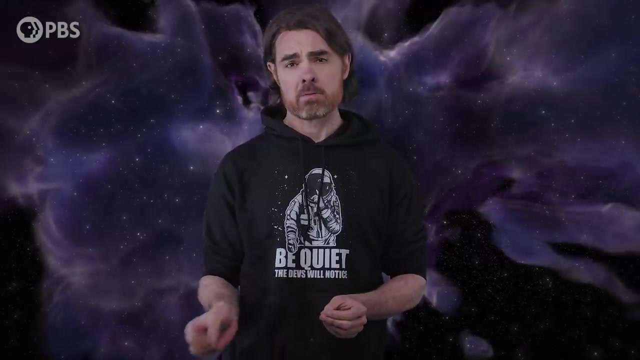 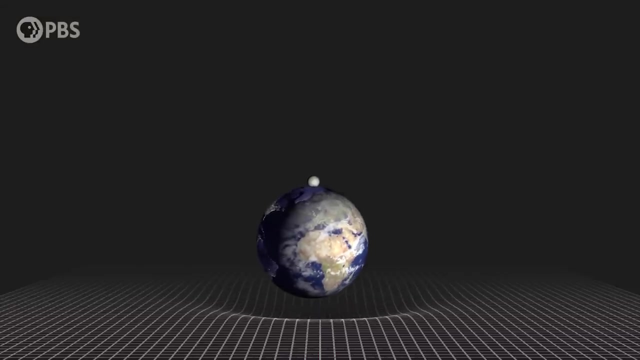 the universe's tendency to disorder. So if you allow that entropy to hold you in your seat for a bit, I'll tell you all about it. Gravity is the odd one out among the fundamental forces. It's enormously weaker than the other three and it's also not a quantum force, At least it's not in general relativity. 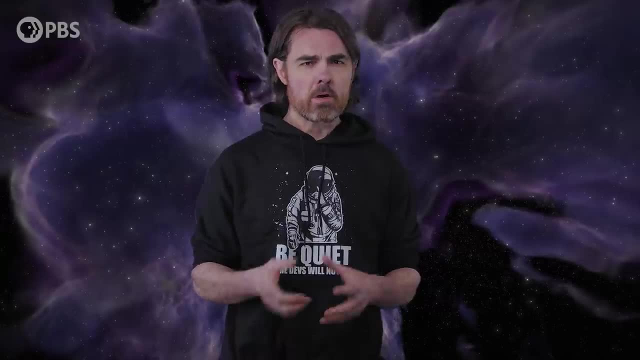 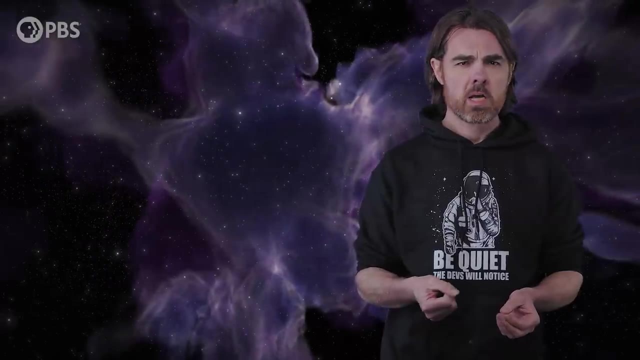 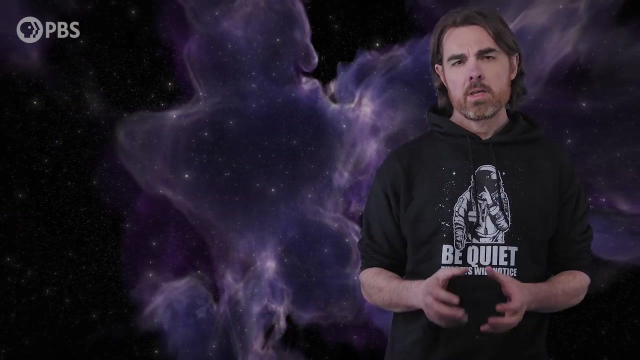 our best description of gravity. And gravity has steadfastly resisted our century-long effort to quantize it, to unify it with the other fundamental forces. But what if that's not the case? That's because gravity isn't quantum, In fact, what if it's because gravity isn't even fundamental? 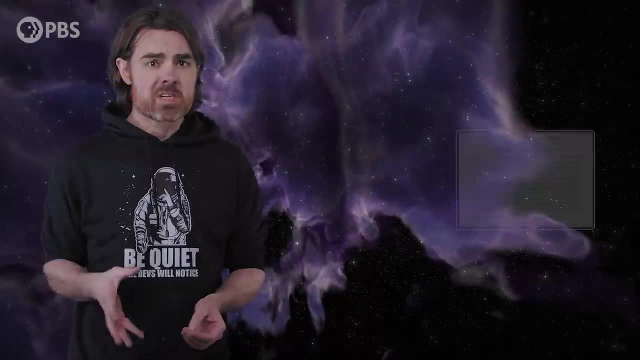 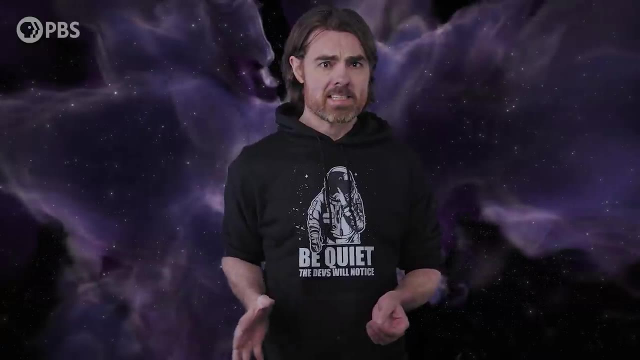 There are a number of proposals along this line, including the buzzy recent work by Jonathan Oppenheim, but we're going to have to come back to that, Because there's an idea that you've been asking us to cover for years now. That's the emergent entropic gravity. 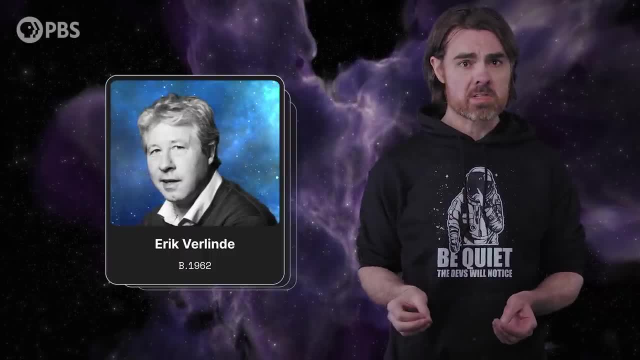 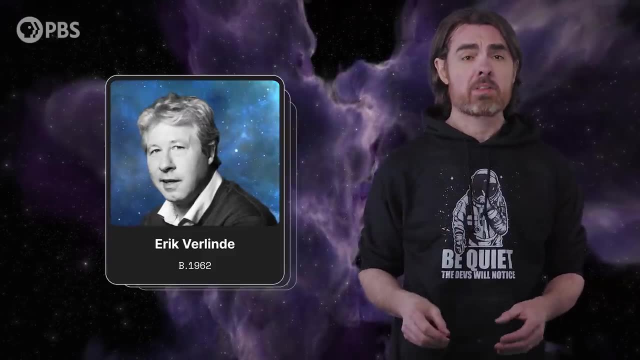 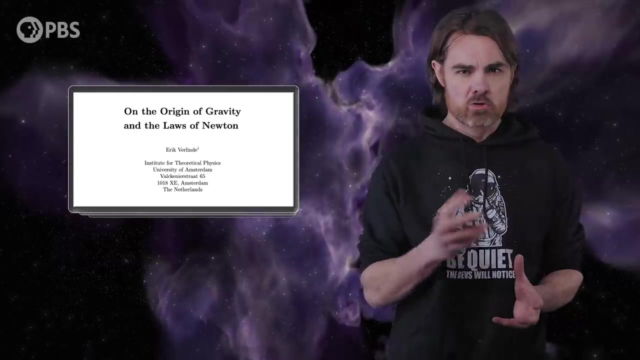 of Dutch physicist Erik Verlinde, who tells us that it's not some fundamental force or the curvature of spacetime that's keeping you in your chair right now, but rather the rise of entropy on the boundary of the universe. Today, we're going to lay out the basics of Verlinde's entropic gravity, as it was published. 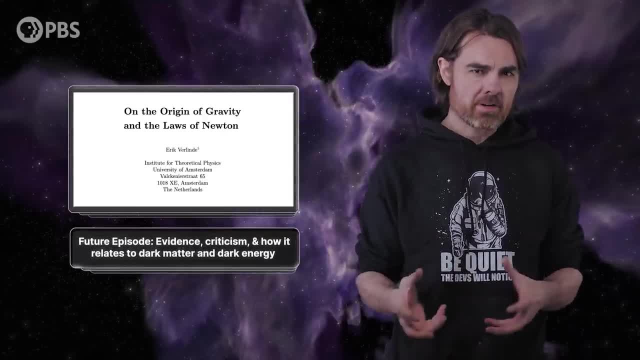 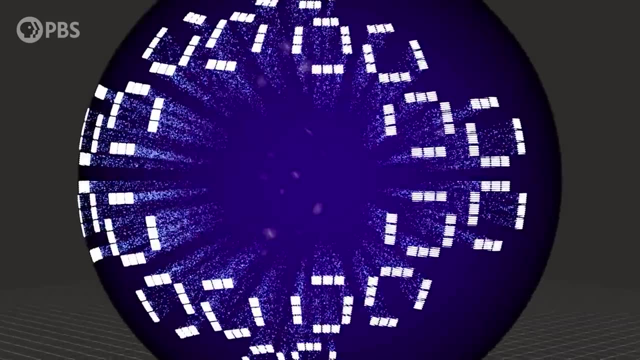 back in 2010.. We'll follow up with an episode on the evidence and the criticism and what the idea has to say about dark matter and dark energy. This episode follows directly from our last one, where we explored how space can emerge as an inward projection from its infinitely distant 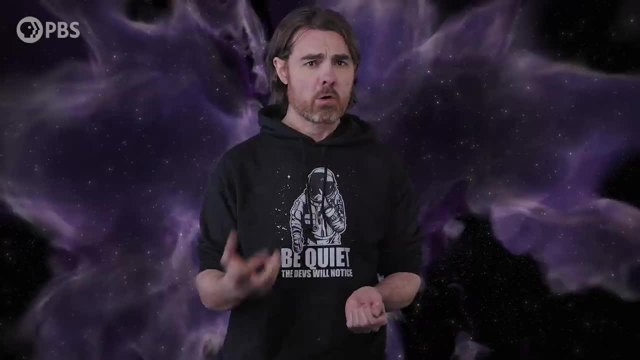 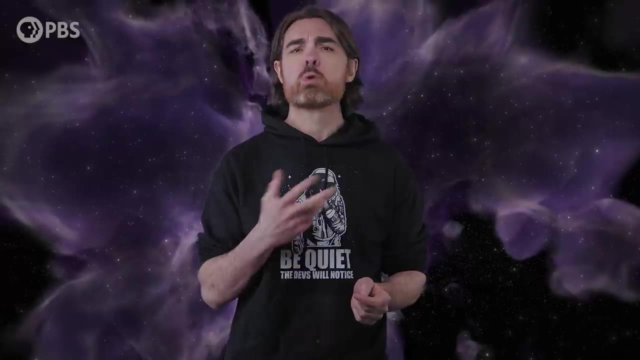 boundary through the holographic principle. A lot of what we talk about in this episode is about the dark matter and we'll draw from that episode, so it might not be a bad idea to check it out. But let me recap anyway to emphasize the most important stuff. I'm also going to sprinkle in 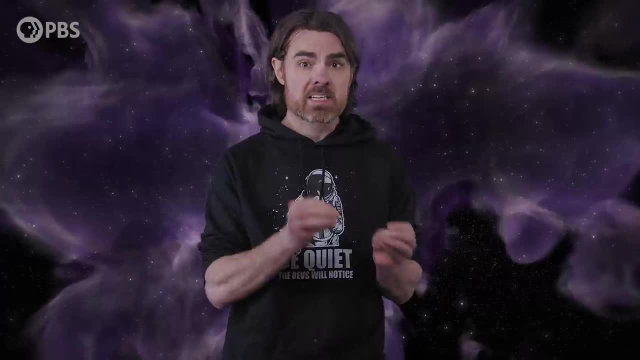 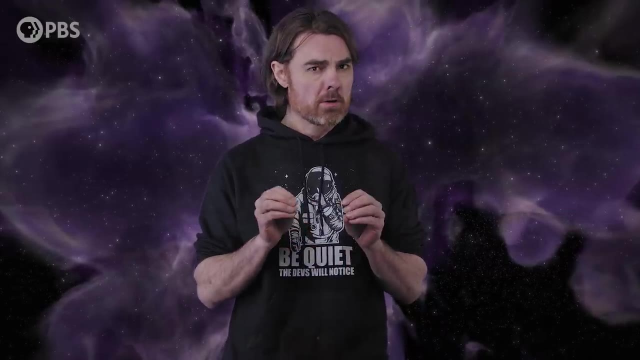 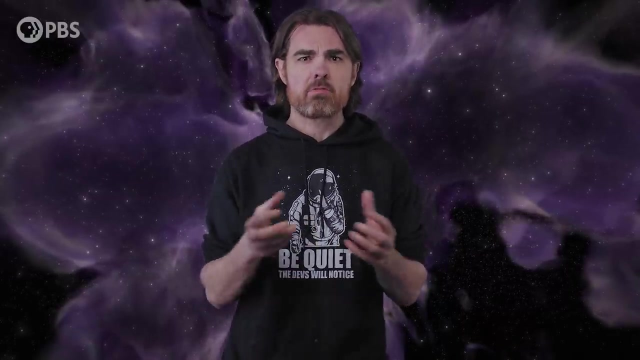 a bit of math and we'll use that to construct Verlinde's ideas. But if the math isn't your cup of tea, relax, I'll give you everything you need to follow with normal human words. So the holographic principle grew out of black hole thermodynamics, from the fact that the 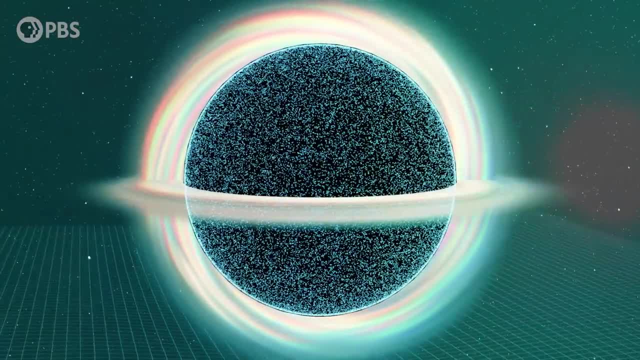 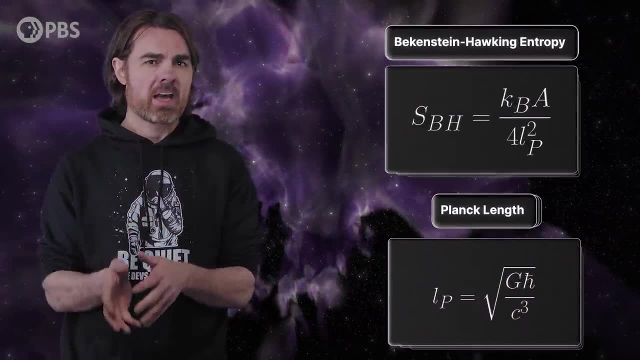 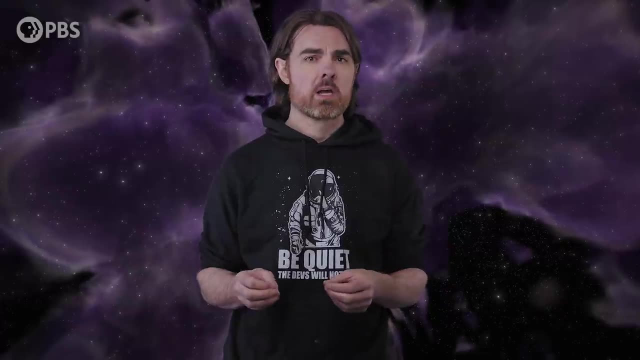 information that can fit inside a black hole is proportional to its surface area. That information is hidden from the outside world, so this also gives the black hole an entropy given by the Bekenstein-Hawking formula. It turns out that the same information limit applies to all of space. 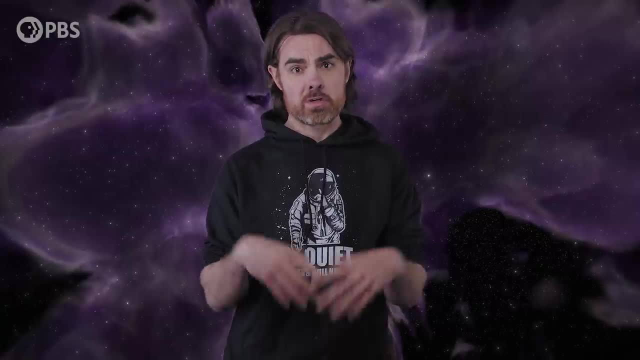 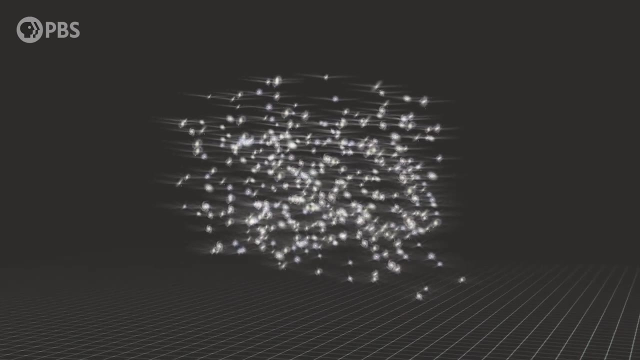 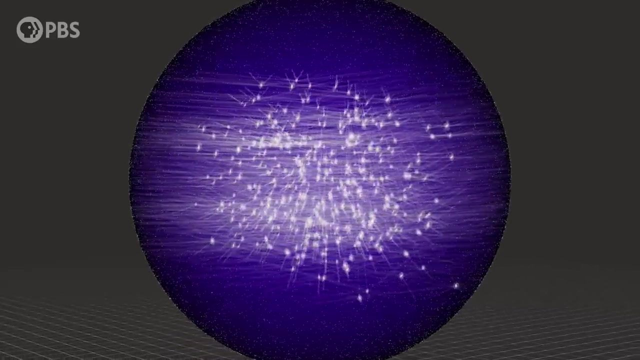 so that it's in principle possible to encode the contents of a universe on its boundary. In fact, according to the holographic principle, the particles and fields and gravity and laws of govern our universe also play out in lockstep on its infinitely distant but infinitely compacted. 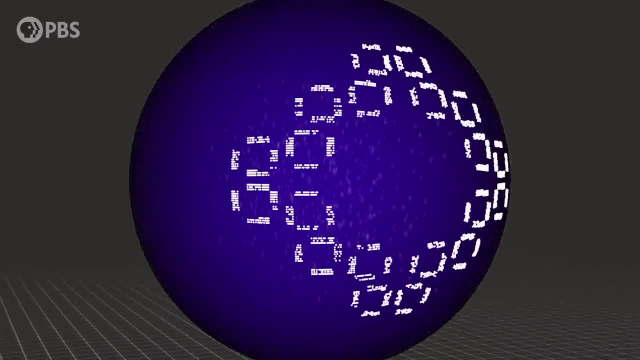 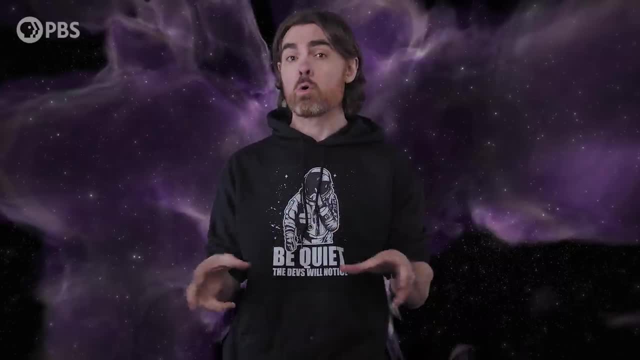 boundary. On that lower-dimensional, gravity-free boundary, a very different set of laws encode everything that happens on the interior. The boundary encodes what we call the bulk, and perhaps vice versa. The only concrete mechanism for this that's currently known is: 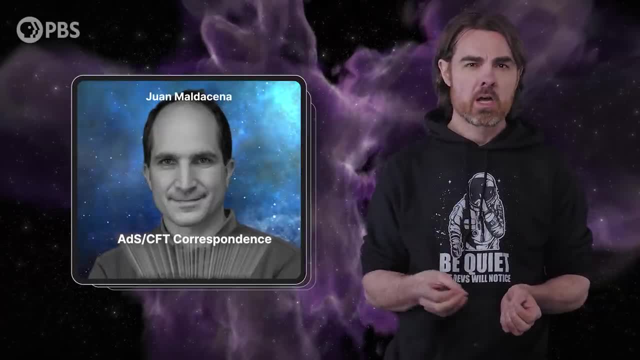 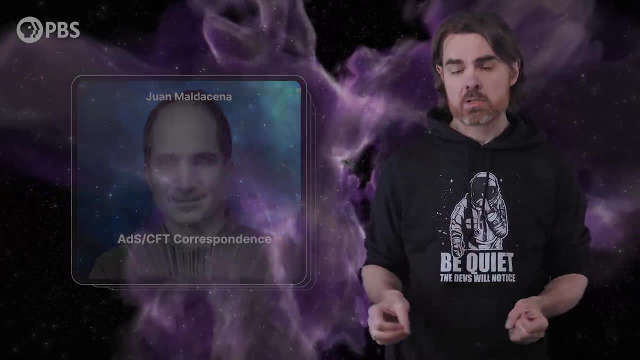 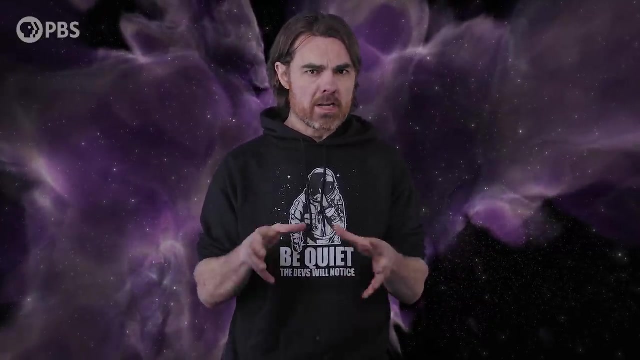 Juan Maldacena's ADS-CFT correspondence, which unfortunately doesn't quite apply to our universe. Still, it's a strong lead that there is a version which does. In ADS-CFT the interior space, the bulk contains a string theory and gravity emerges within that. 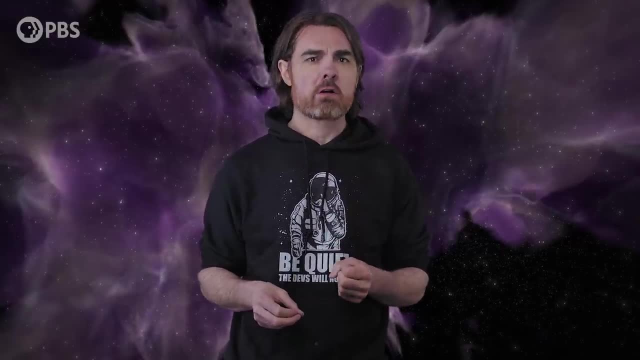 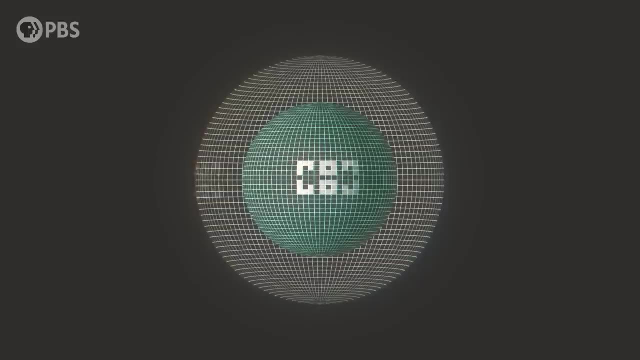 string theory. But we don't need string theory to see how gravity might be a natural prediction of the holographic principle. Last episode I showed you a scheme by which this X-ray of the holographic principle would work. The X-ray dimension can be encoded in the scale of structures on the boundary. 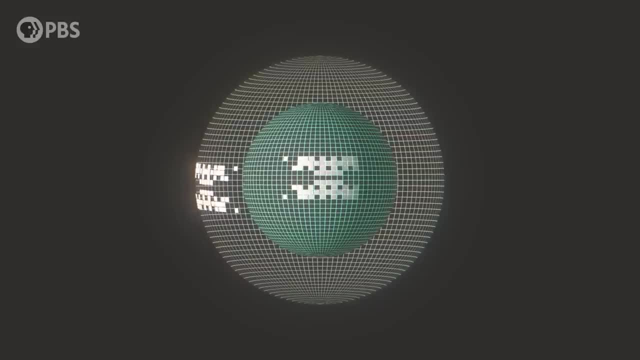 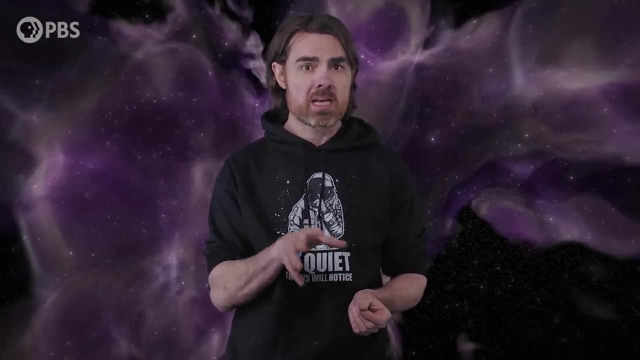 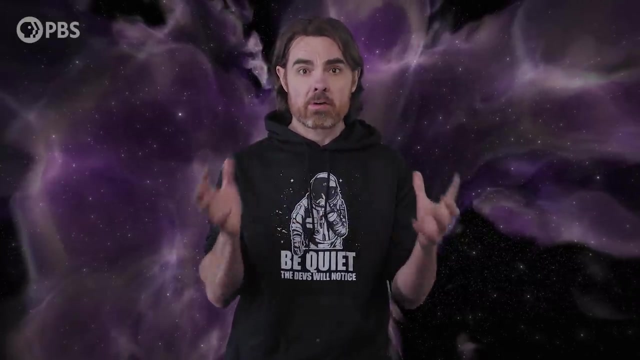 with larger structures on the boundary manifesting as structures closer to the center of the bulk. Today we're going to explore one idea for how gravity can also emerge within that space as a statistical side-effect of the interplay of… whatever it is that's happening out there on the 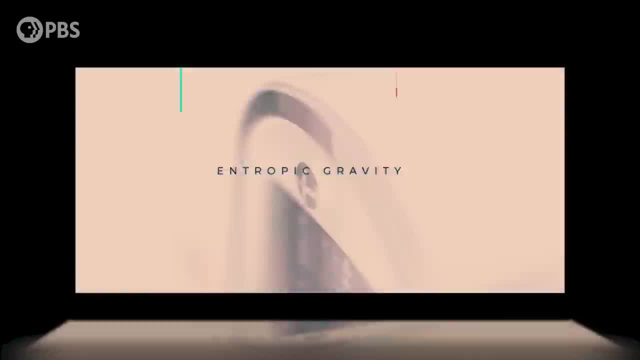 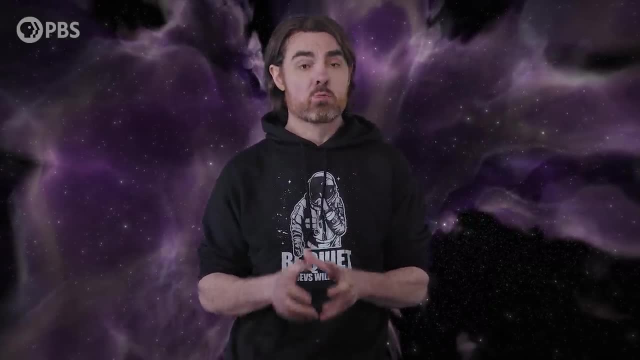 boundary. This is the entropic gravity of Erich Wallinder. Entropic gravity is by no means broadly accepted, but it's not the only thing that's happening in the boundary. This is the entropic gravity of Erich Wallinder. It is taken seriously by reasonable physicists. After all, there is a 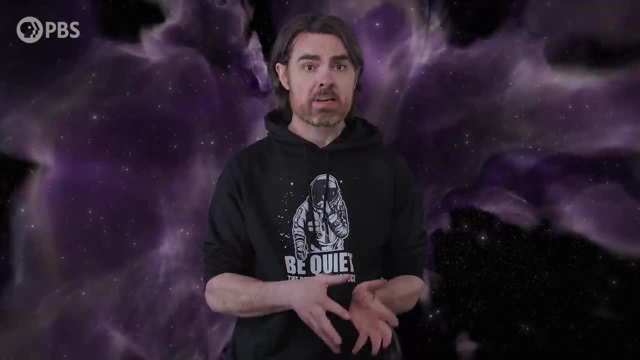 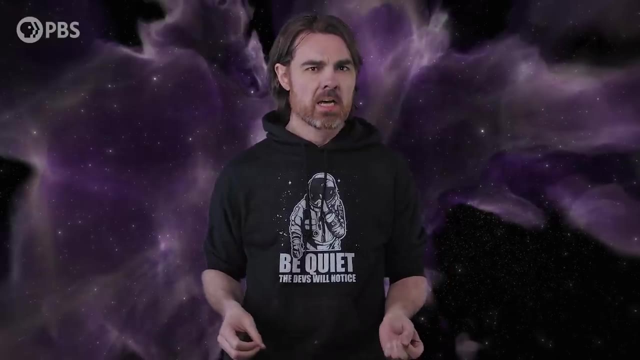 fascinating and still mysterious connection between gravity and entropy, as Bekenstein and Hawking discovered. And there's a fascinating neatness to Wallinder's idea that seems like it's telling us something, even if it isn't the whole picture and maybe even if it's wrong. 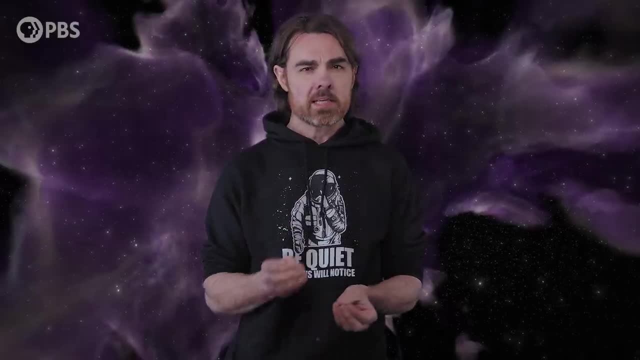 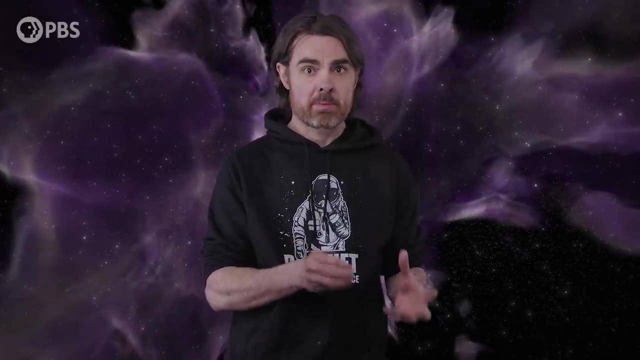 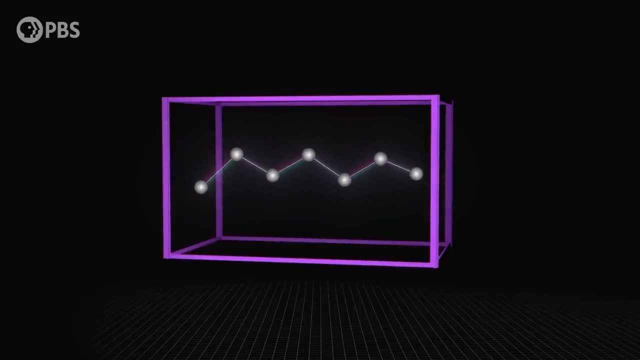 To understand how gravity might arise entropically, let's think about a less… out-there system. We'll use the same thought experiment that Wallinder uses in his entropic gravity paper. Imagine a long molecule that is free to move and fold in any direction. We place it in a box of constant temperature with. 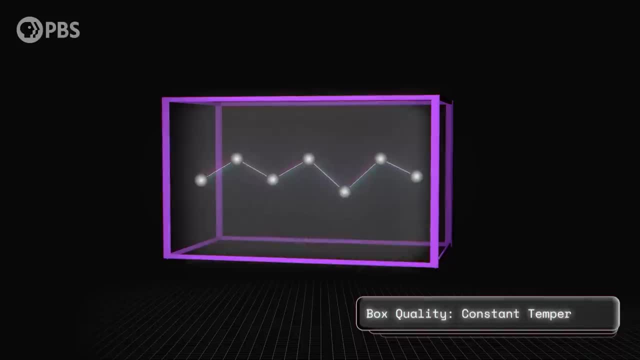 one end fixed to the wall of the box. If we ignore any possible external forces acting on the molecule, we might expect it to just curl up. This is because of all the ways the molecule could move. it's far more likely to end up in a coiled configuration than remain straight. This is 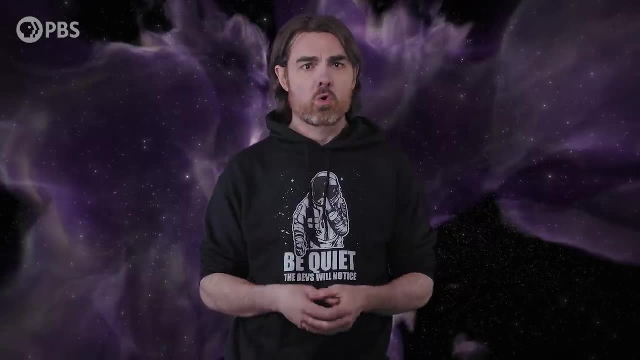 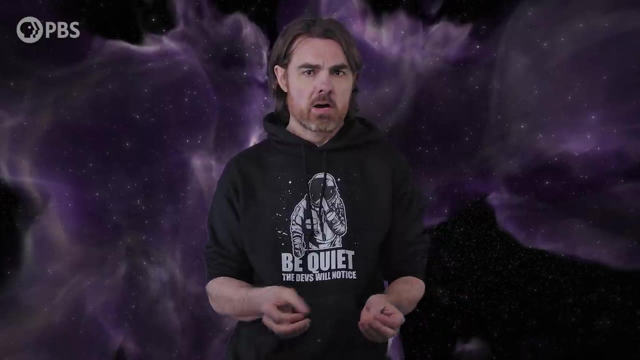 one way to think about entropy. The molecule will almost always take a more probable, higher entropy configuration of being curled up, because there are way more configurations, or what we call microstates, in which the molecule is curled compared to it being straight. 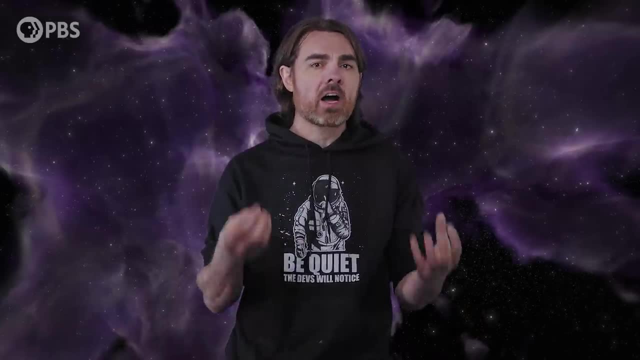 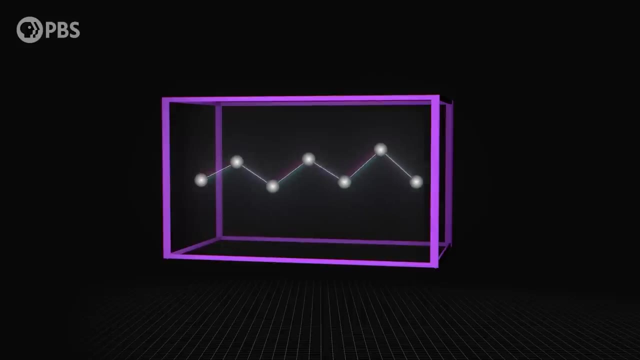 Being in one of the many random coiled states is a higher entropy configuration than the very few straight states. If we straighten the molecule, we have to exert a force and expend some energy to do so. If we let go, it'll curl up again. because there's an effective force pulling it back. I should add that there's nothing magical going on here. The molecule shares its temperature with the air in the box. the atoms have randomly oriented vibrations and are being randomly smacked by air molecules, and these will pull and push the molecule towards random configurations. 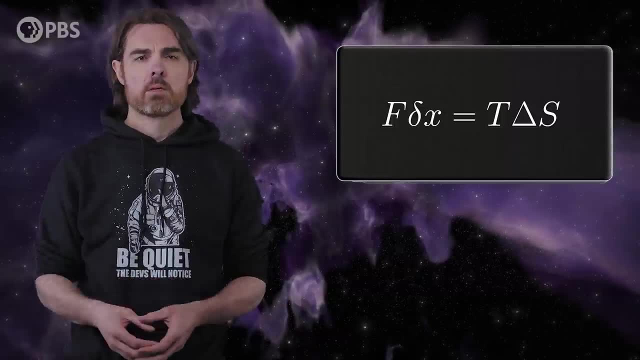 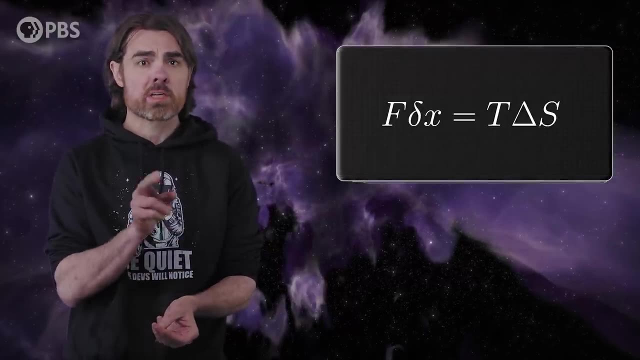 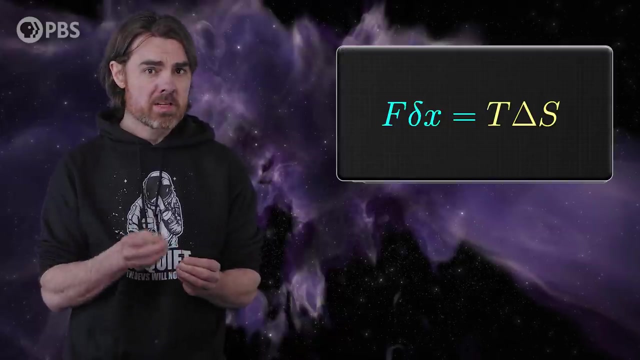 which are overwhelmingly the coiled ones. There's a simple relationship between the force required to pull the molecule or the entropic force that the molecule exerts on you. This is really saying that the amount of energy, the force times the distance pulled is equal to the temperature of the system times the change in entropy after that little motion. 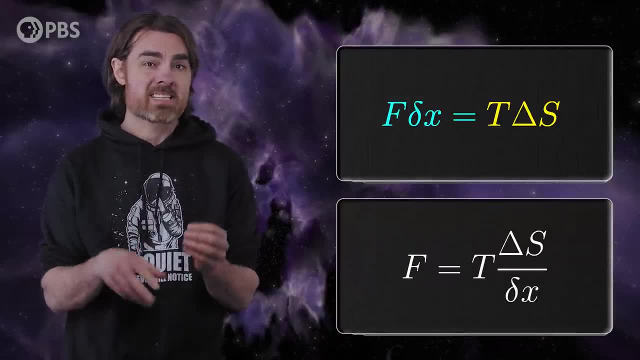 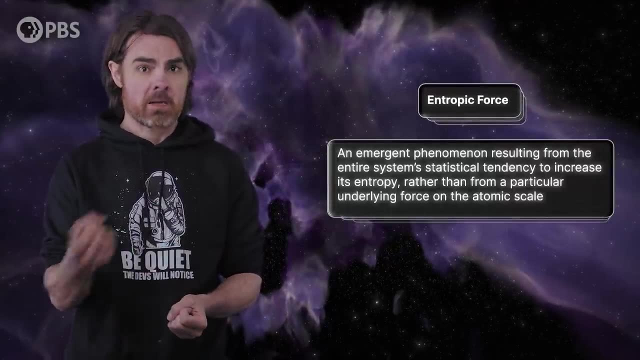 happens, Or that the force is equal to the temperature times, the entropy gradient, And we call this an entropic force. It's exactly what you experience when you pull on an elastic band, In fact, any time you have the movement of matter in the service of. 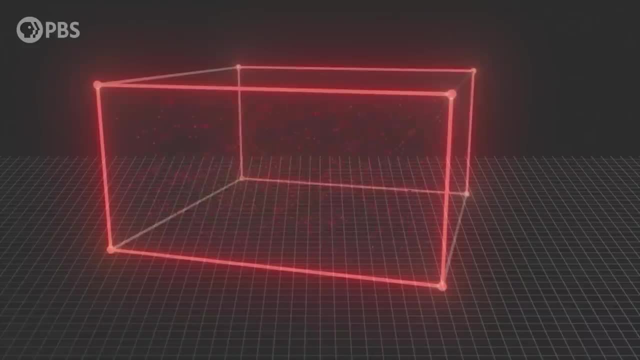 increasing entropy. there's an entropic force. For example, if you force all the air in a room into a box and then release it, it'll rush to fill the room and generate an enormous entropic force in doing so. The proposal of Eric Valinde is that gravity is also an entropic force. 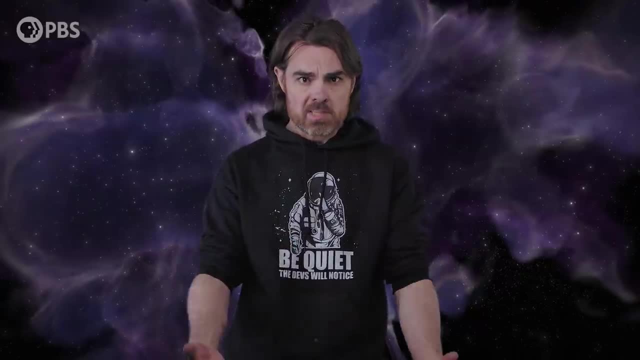 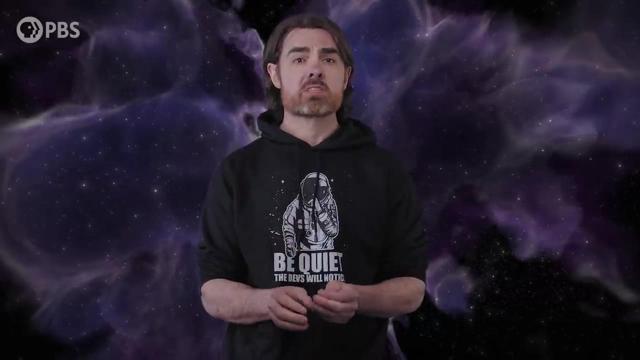 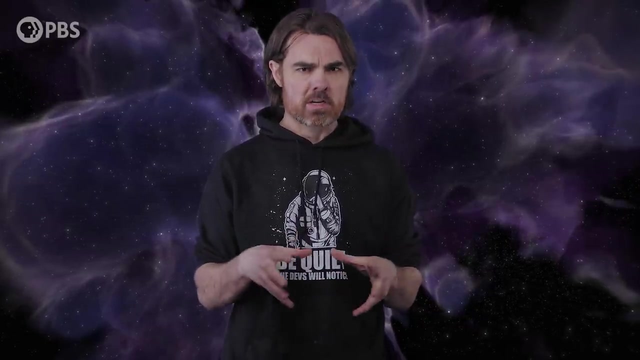 At first glance that seems odd. Gravity is a property of spacetime itself. Even empty spacetimes are. what exactly is pushing or pulling in empty space? Valinde constructs his argument in the context of a holographic universe in which at least one dimension of space is also emergent. He argues that the entropy of the stuff on the holographic 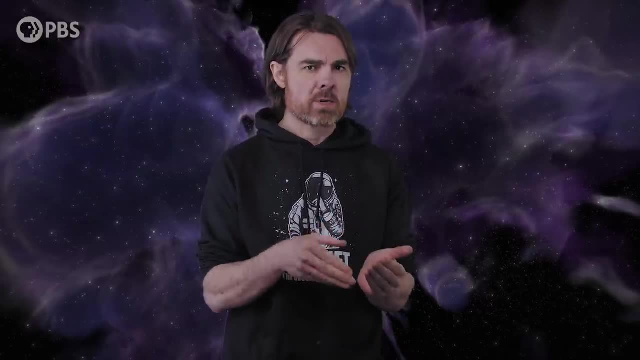 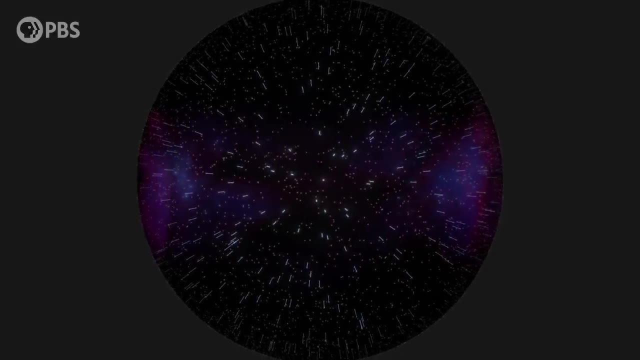 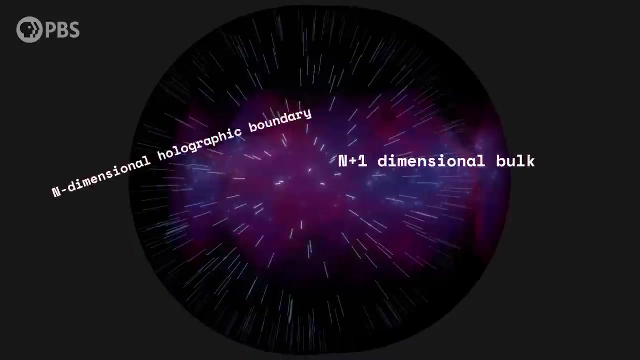 boundary must increase and that rising entropy manifests as gravity in the interior. To build up this idea, we're going to need to keep in mind dual pictures- Something is happening on the boundary and something is happening in the bulk- And they encode the same thing, even if 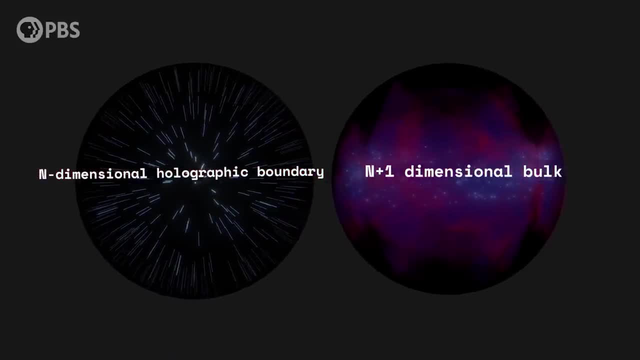 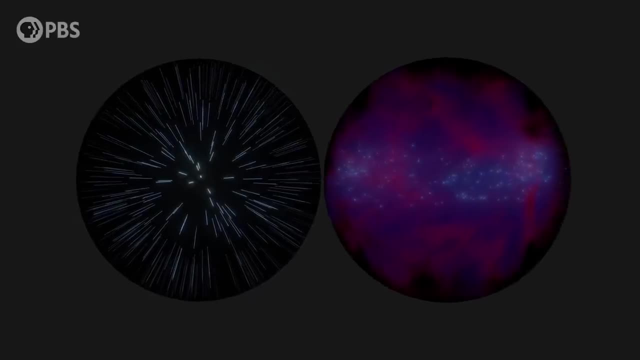 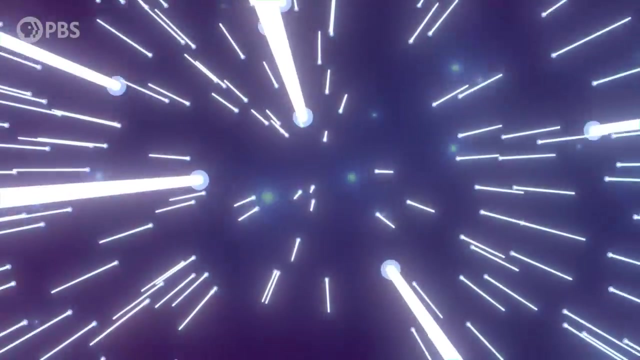 they sit very differently in our mental imagery. We will flip between them as convenient and even merge them slightly, But remember that these are two distinct ways of describing the same system. Ok, so somewhere in the bulk of a holographic universe we have a star with some mass. 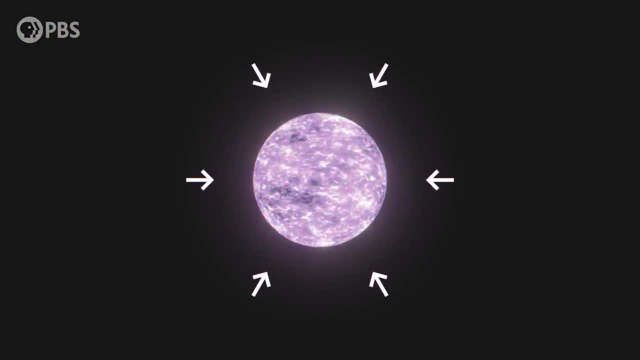 Let's see if we can figure out the gravitational force produced by the star without ever using any theory of gravity, just by visiting the boundary To derive such a law. we want to know how much gravitational force is felt at different distances, So let's imagine a series of spherical surfaces. 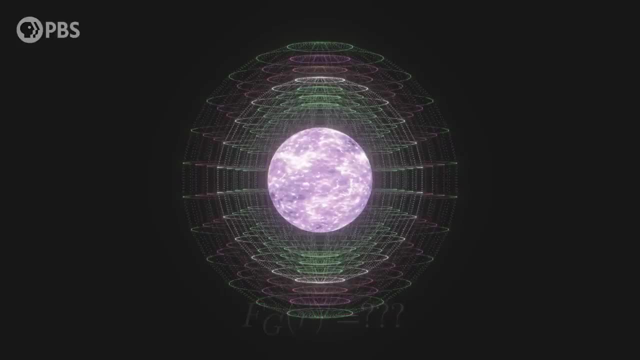 around the star. Let's imagine a series of spherical surfaces around the star. Let's imagine a series of spherical surfaces around the star. If the star is massive and compact enough, then one of these surfaces would be an event horizon and we'd actually have a black hole. 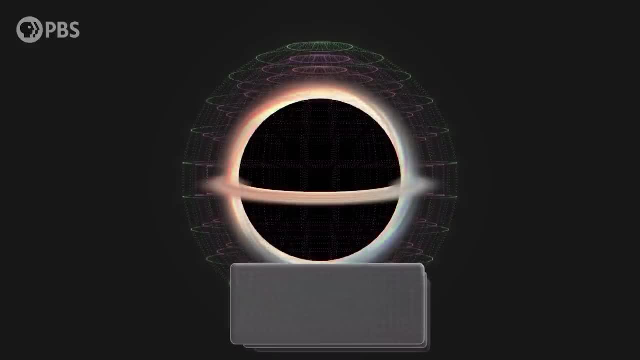 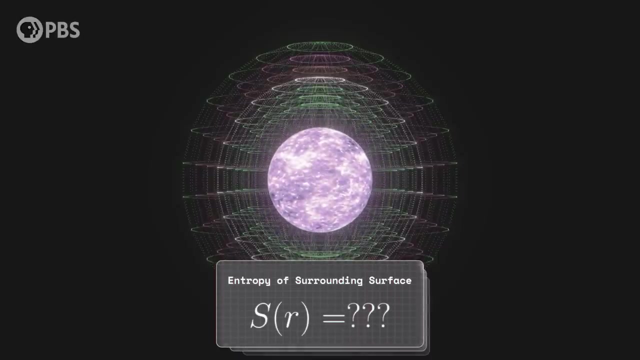 Then the entropy of that surface would be the Bekenstein-Hawking entropy. Basically it would represent the amount of information of everything that previously fell through that surface. But even if this surface isn't an event horizon, we can give it an entropy. It's also the entropy of everything interior to that. 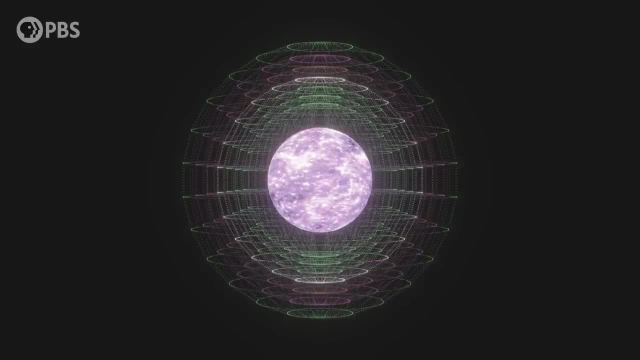 surface. But that makes the most sense if we zip out to the boundary. If this is a holographic universe, then the particles on this surface map to the boundary. In fact, the particles on surfaces of all sizes map to the same boundary and play out together. 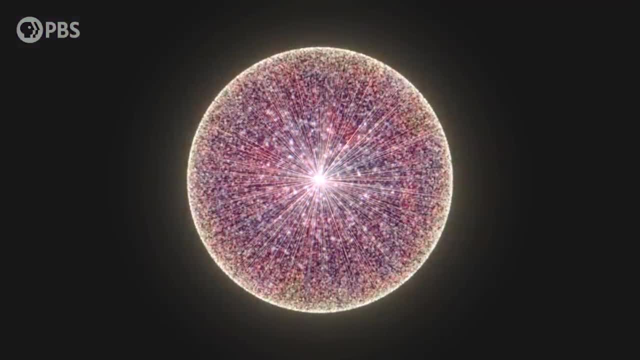 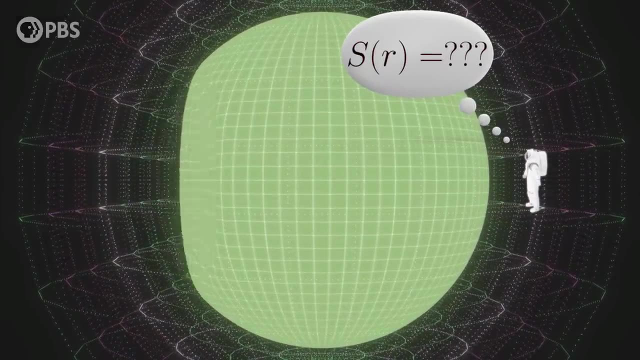 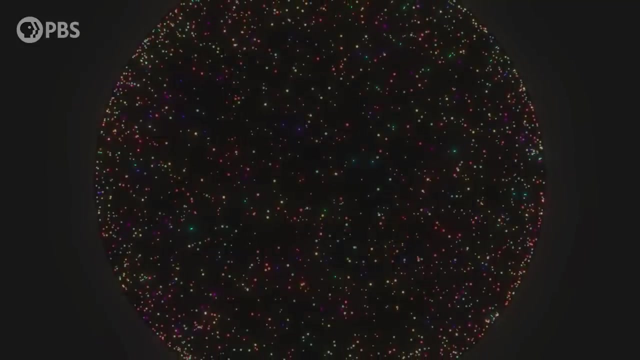 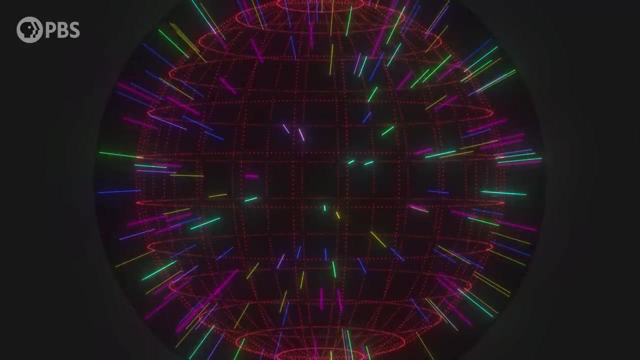 overlapping in that lower dimensional space. We want the entropy of this one surface with respect to someone outside that surface. That translates to how much information is hidden within that surface. Let's start with the holographic boundary from which our bulk universe emerges. Imagine that it emerges from the outside in. That's not really the case, but it helps us. 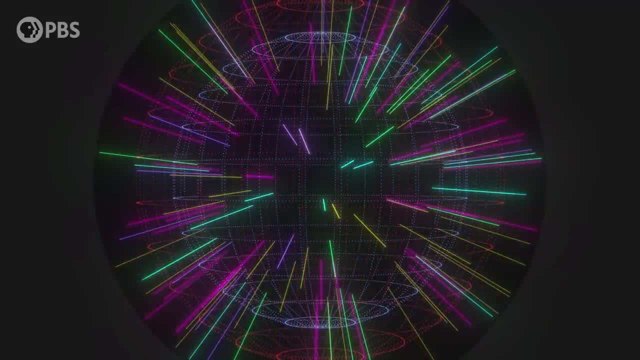 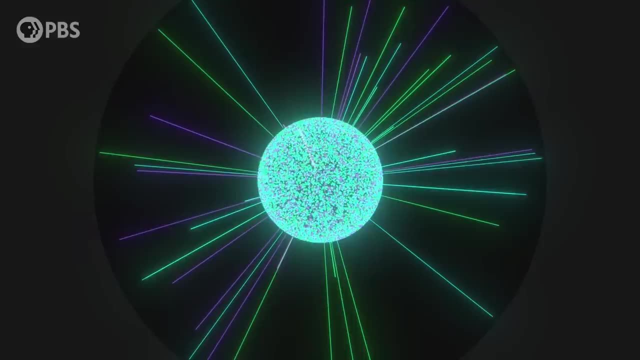 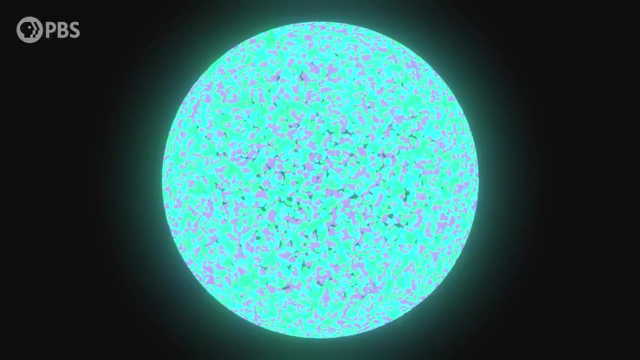 represent this visually. We're going to partially emerge our universe down to this one surface, so we can depict a special subset of the boundary as actually lying on this surface. in the bulk, This is the part of the boundary that corresponds to everything below this surface. So from now on, when I say boundary, I mean the component of the. 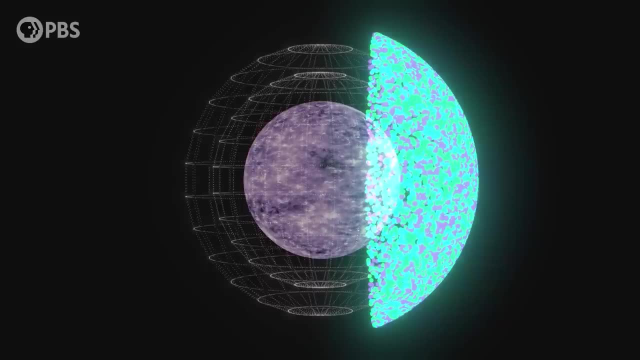 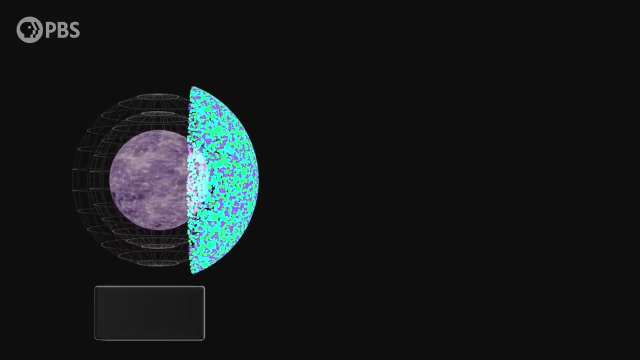 holographic boundary corresponding to the region of the bulk enclosed by this surface. OK, hold on for just a little bit of math. We know that this surface contains a mass, so we can say that it also contains energy. by Einstein's, E equals mc squared, That's the energy. 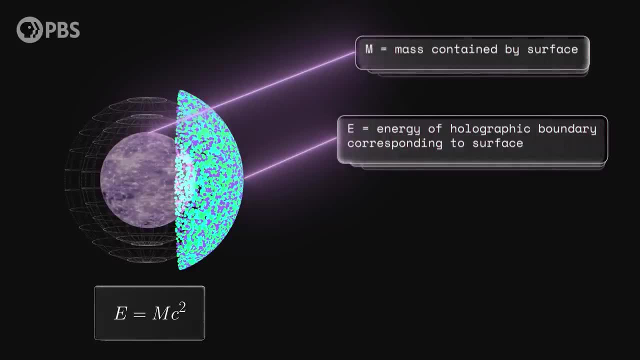 of the interior, but it also has to be the energy of the corresponding holographic boundary. We can also give that boundary a value of 0, which is the energy of the interior. We can also give that boundary a temperature, assuming the stuff on the boundary is in thermal. 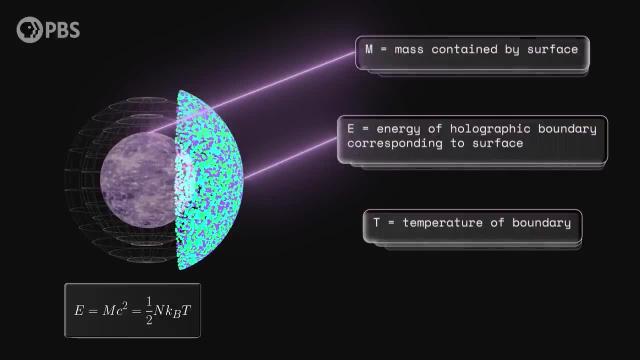 equilibrium, so that that energy is evenly spread over all possible states And that n-thing is just the number of possible states on the boundary and the total number of arrangements of particles inside the volume. that would give you the particular values of energy mass and temperature. 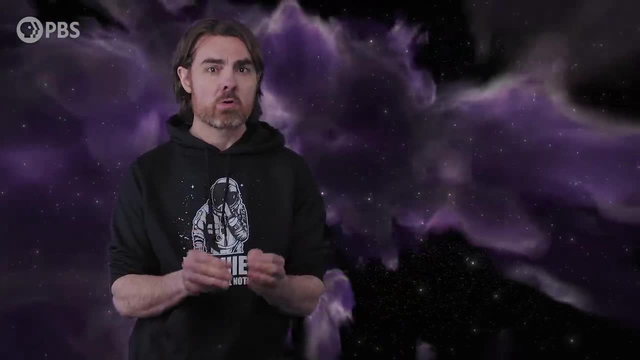 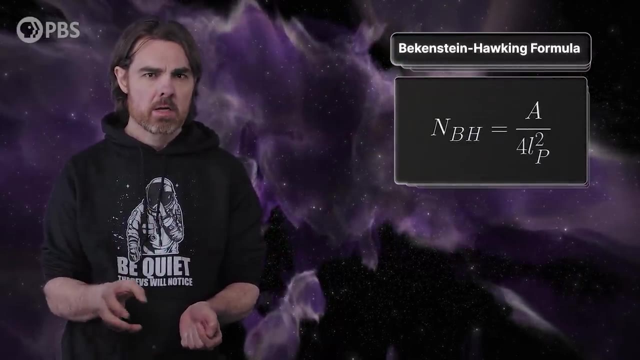 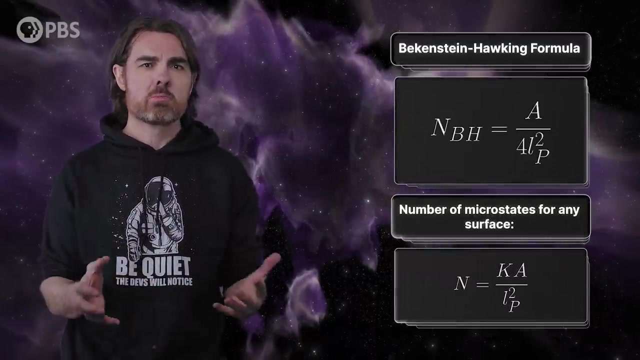 But that also corresponds to the amount of hidden information within the surface. It's entropy. We know the maximum value for this: It's the Bekenstein-Hawking entropy. so the number of Planck length squares over that surface. For our surface, let's just assume that the entropy and n are still proportional to the. 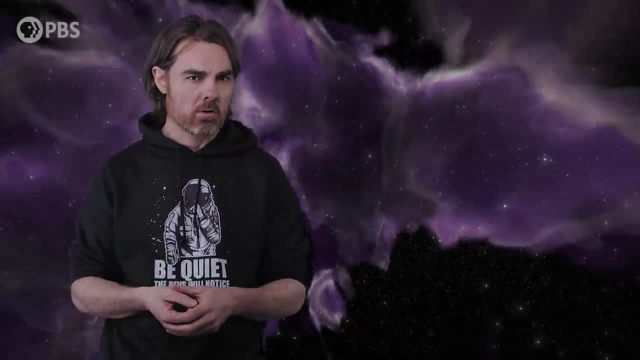 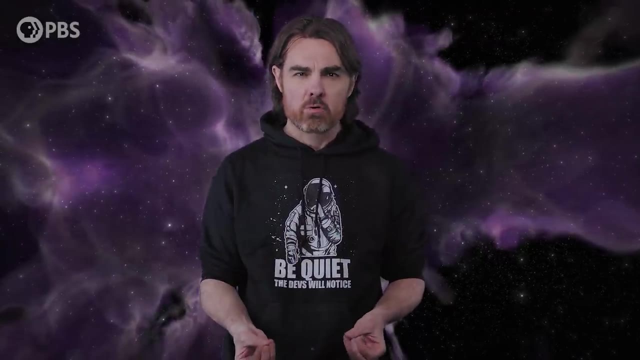 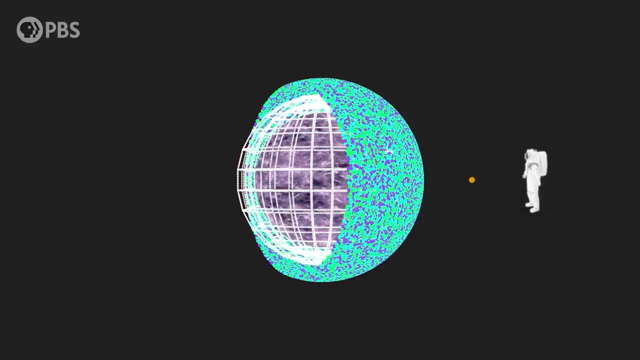 surface area, but presumably smaller than for a black hole. OK, one more step. We want the gravitational force, so we need another particle to feel that force. Let's add a tiny mass and move it close to the surface from the above emerged. 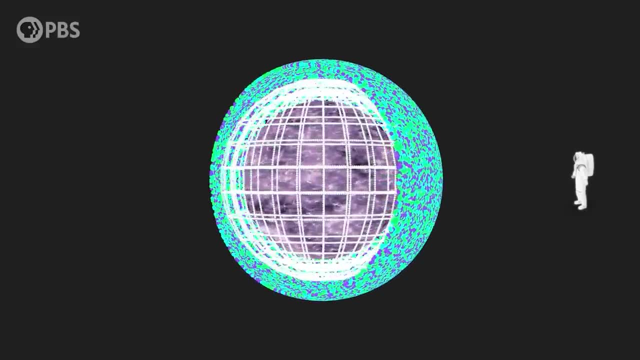 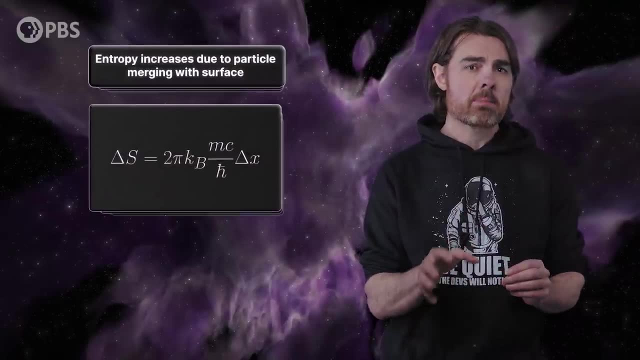 part of space. When that happens, the entropy of the boundary increases, because the information from that object is lost to the external region. The boundary gains the same amount of entropy as dropping something into a black hole event horizon. This equation is just saying that. 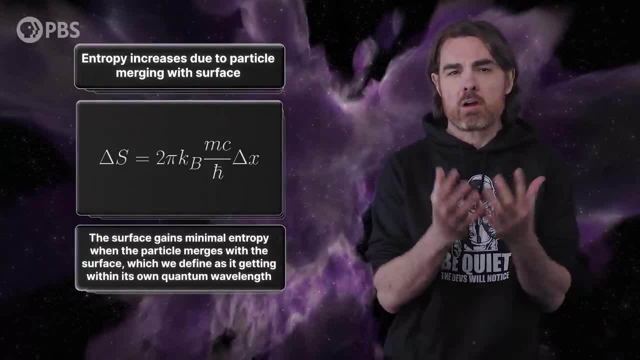 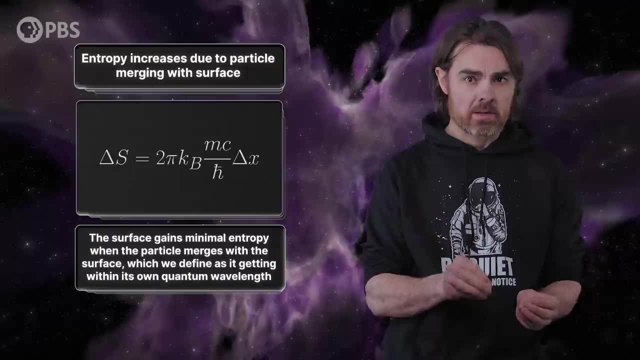 the surface gains minimal entropy, equivalent roughly to a bit, when the particle merges with the surface, which we define as it getting within its own quantum wavelength, in this case the Compton wavelength of the surface. But just like we saw with the coiling molecule, 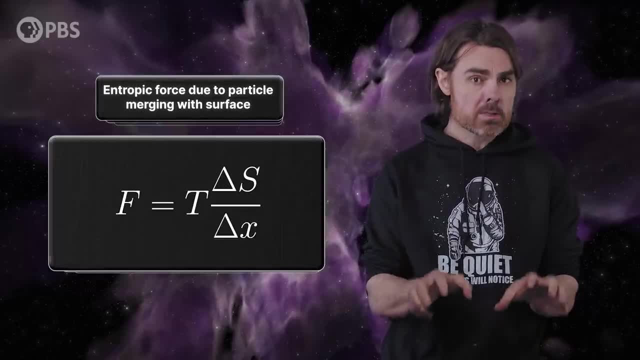 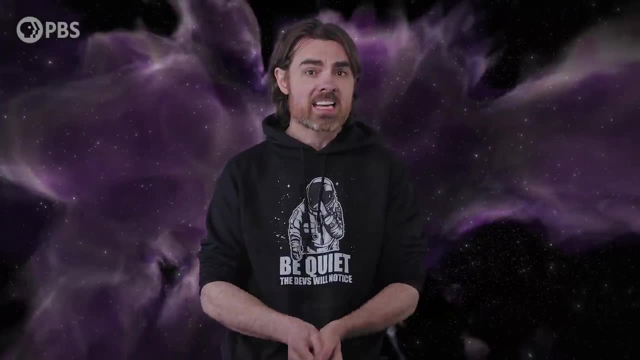 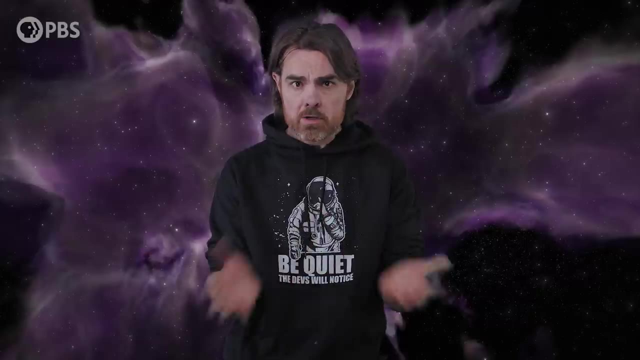 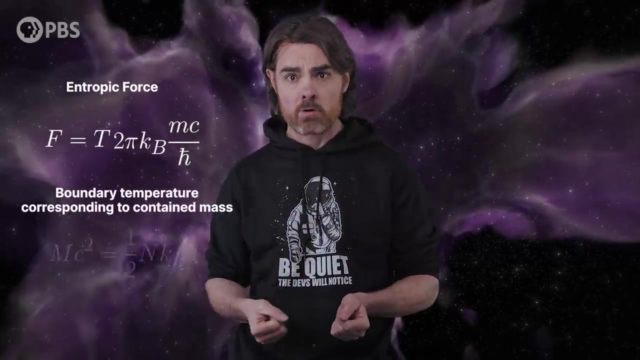 this tiny increase in entropy should have a corresponding entropic force. Whatever crazy interactions are happening out there on the boundary, they are statistically inclined to bring our particle closer to this surface because that motion increases entropy. If we bring everything together, the delta s over delta x from dropping a particle through the horizon. 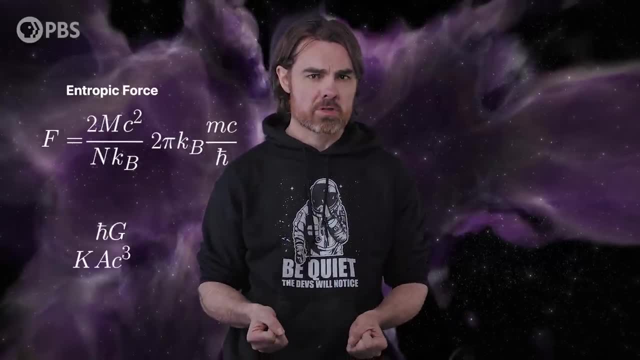 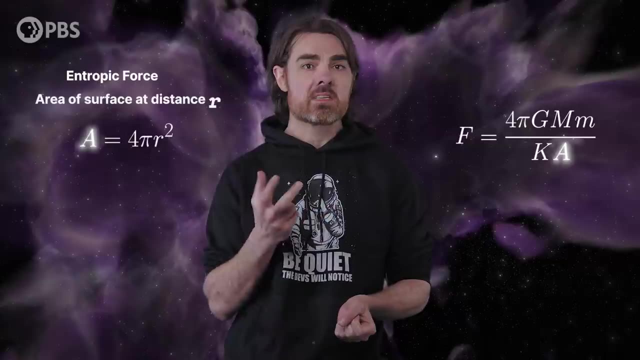 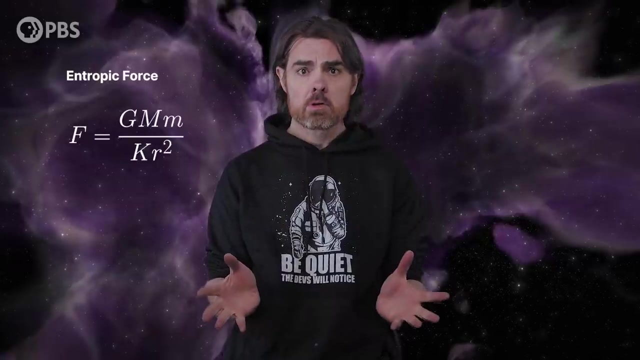 and the temperature from the overall entropy of the surface. all the h-bars and the c's and the kb's cancel out and we replace the area of the sphere with 4 times pi times its radius squared and we see that the algebra shakes down to Newton's universal law of gravitation within some constant. 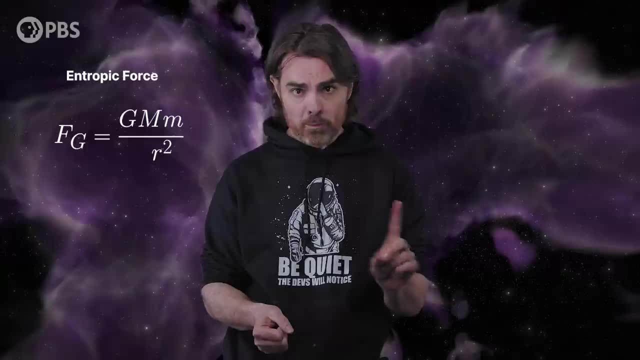 And if that constant is 1, because we got our surface entropy formula right, then we have Newton's exact equation. If we have the formula, then we have Newton's exact equation. And if we have the formula, then we have Newton's exact equation. 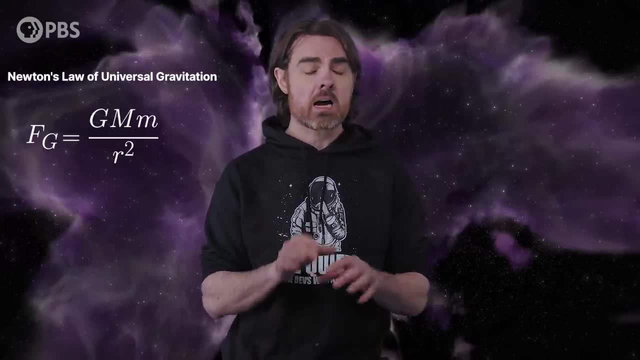 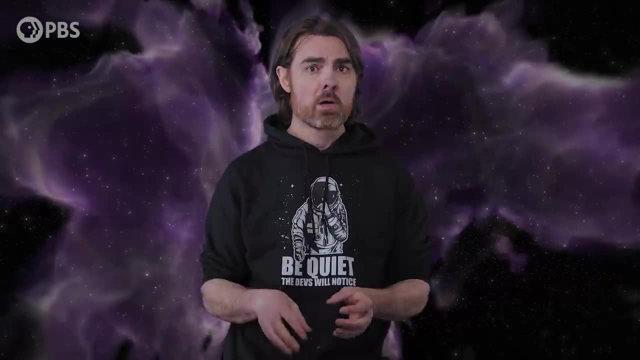 And if we have the formula, then we have Newton's exact equation. And if we have the formula, then we have Newton's exact equation. We just derive Newtonian gravity with arguments that are entirely thermodynamic. This is basically saying that if objects in the bulk move in such a way as to maximize 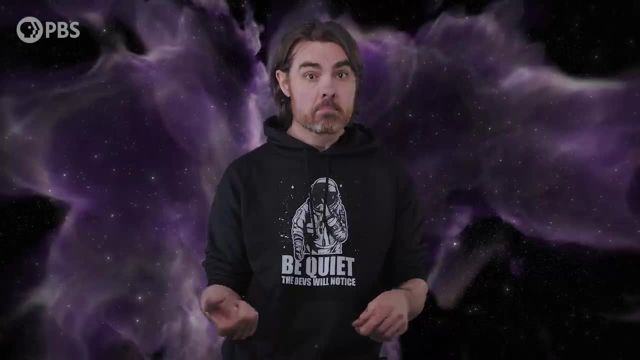 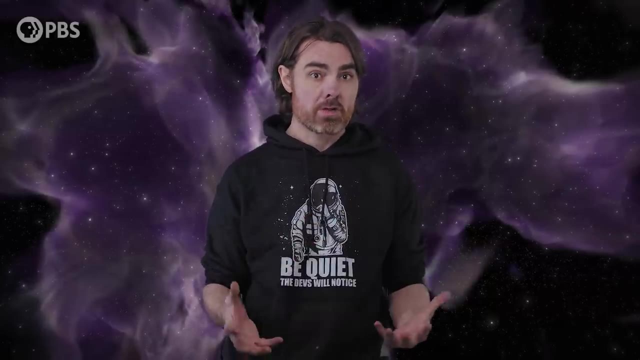 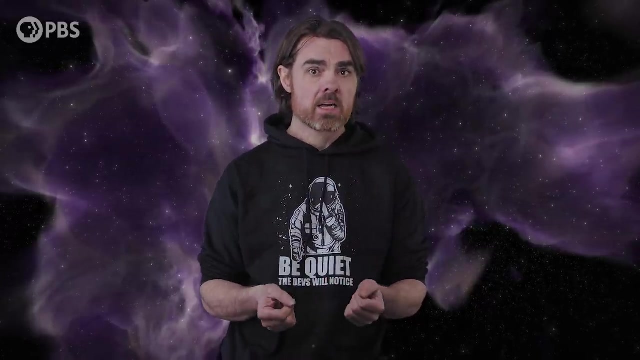 entropy on the boundary, then that motion means falling towards other masses in the bulk. Remember that Hawking and Bekenstein used gravitational theory and quantum mechanics to get black hole thermodynamics. But entropic gravity turns on its head. It starts with thermodynamics and finds that gravity just falls out. 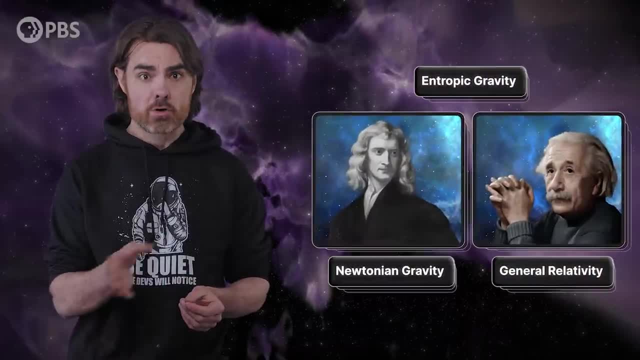 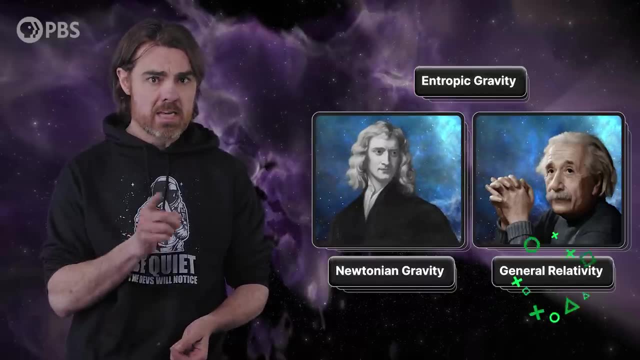 But let's not get ahead of ourselves. Firstly, this is just Newtonian gravity. Can entropic gravity reproduce Einstein's general relativity? Well, in the 2010 paper, Verlinde argues that yes, it can, although the derivation is a bit.